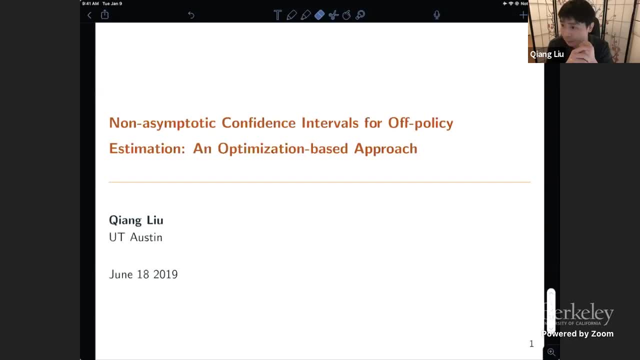 confidence bounds for off-policy validation. So we'll propose what we call optimization-based algorithm, which is framing the construction of confidence intervals into an optimization problem, and we can apply PIMODU methods to kind of solve it efficiently. We'll see how it goes. 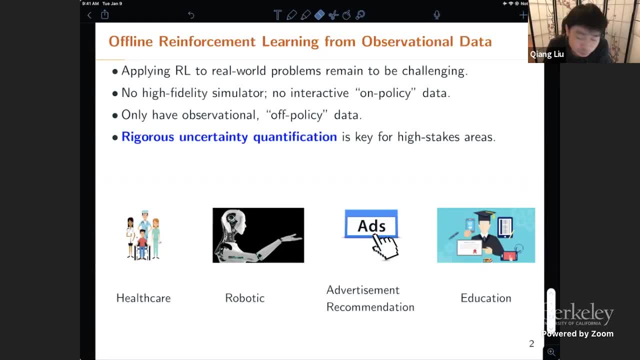 Okay, so I guess I don't need to give a heavy introduction to the safety questions after school's talk. but basically the idea here is that reinforcement learning has been really powerful at cases when we have very good simulators such as video games and AlphaGo, right. But on the other, 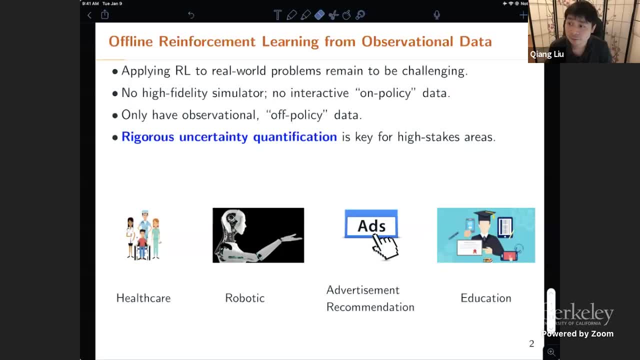 hand, for many real world problems we don't have high-fidelity simulators and we only have observational data right. So this is especially the case where we want to apply reinforcement learning to medical diagnosis education etc. So this is a very high probability case because of the fact that the 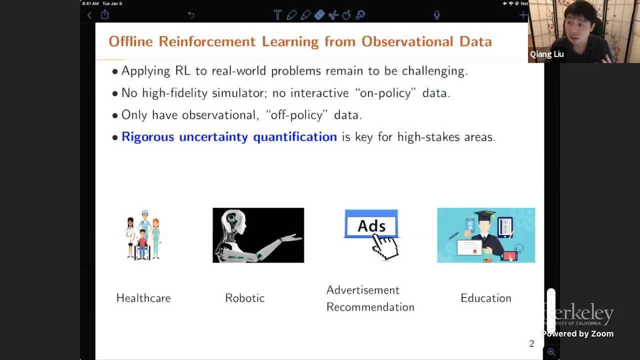 system is very well established, We don't have the right tools to control the response and we're in a very, very high probability case where the robotics, when the robotics, are very expensive and you don't want to damage them. so in these cases, we only have data observed from. 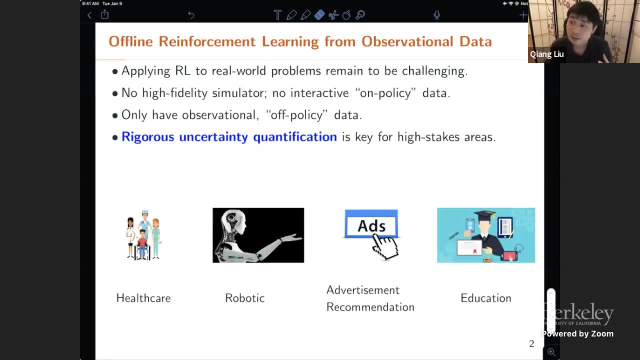 previous experiments, possibly in a very messy, unstructured and unorganized way. right So whether you are doing the right thing, right? So here uncertainty estimation is really important, especially in high-stakes areas such as healthcare. It's actually not enough to just get. 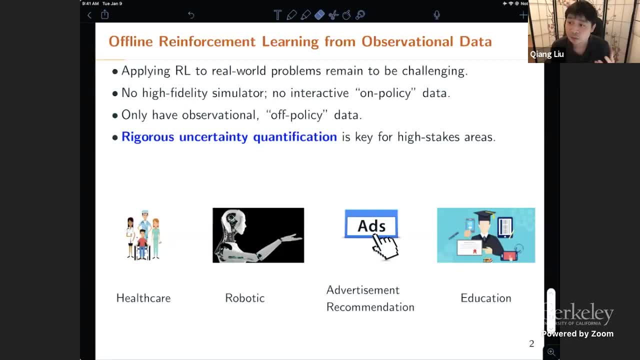 the arbitrary uncertainty estimation. You actually want to make sure that your uncertainty estimation is theoretically verified, It's guaranteed, it's rigorous right. This is why we are motivated to talk about non-asymptotic bounds instead of approximation algorithms. So here's my definition of the problem. 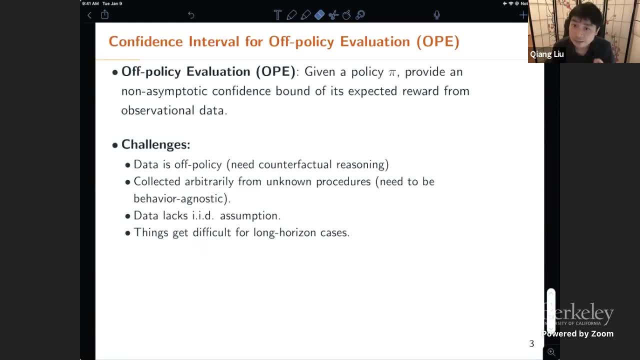 So the problem is that we are given a policy pie and we want to construct a non-asymptotic confidence interval for the expected reward purely from observational data. So there are lots of challenges. First of all, the data is off policy, which means that it's collected from some arbitrary policy. 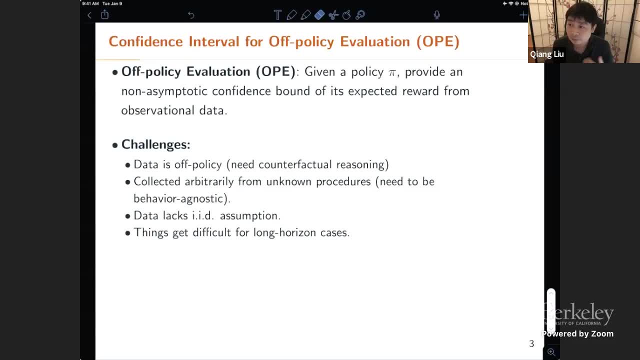 or even no policy right, So arbitrarily. So if you want to reason about a particular pie that hasn't been tested before, it requires some sort of counterfactual reasoning ability right? Another challenge is that the data are collected in some black box way which is unknown to the algorithm. 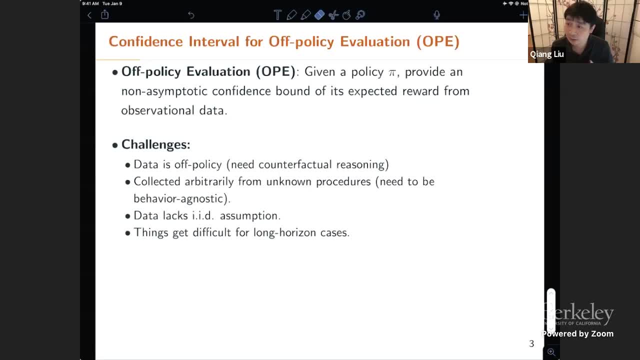 Right. So the algorithm has to be behavior agnostic in order to trade that into account. right, And also, as we are doing, reinforced learning. we have long trajectories And the trajectories are dependent with each other for the time, So we don't have the idea that we have to use the problem. 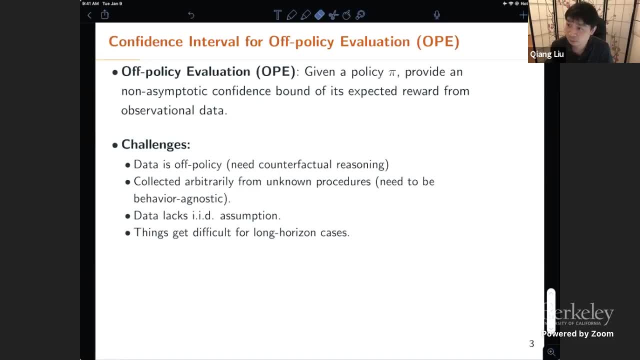 assumption. that was very nice for super-high learning, but here we really don't have that And this actually caused a very strong difficulty for constructing non-eisenstein bonds right. And also that's something called a curse of horizon, which means that if you are reasoning, 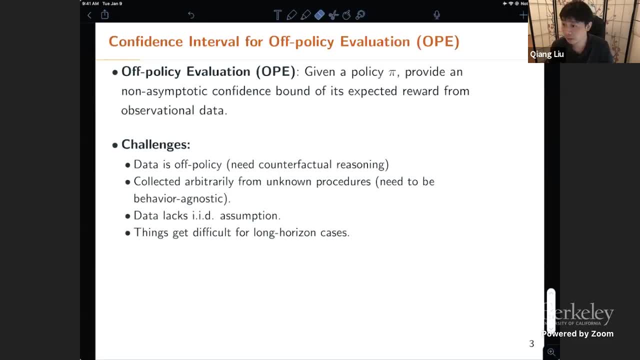 about non-horizon. if your decision making has lots of steps, it's very difficult to reason about the future rewards just because you are considering reasoning multiple steps. Mathematically, it turns out this is also very difficult for traditional methods, right? So these are kind of challenging. 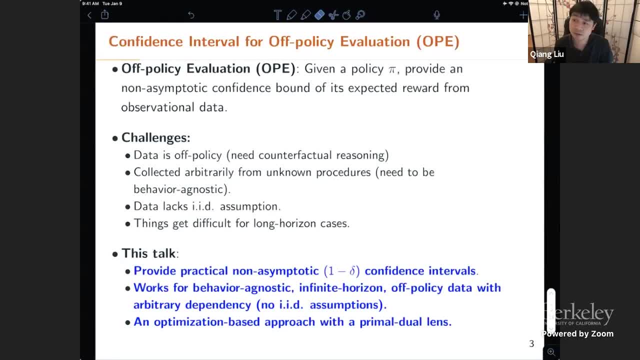 problems, But more or less we actually propose an algorithm I think quite nicely, surprisingly solve all these problems. So we provide a non-eisenstein bound has guarantees and its behavior agnostic works for infant horizon. its off policy actually works for 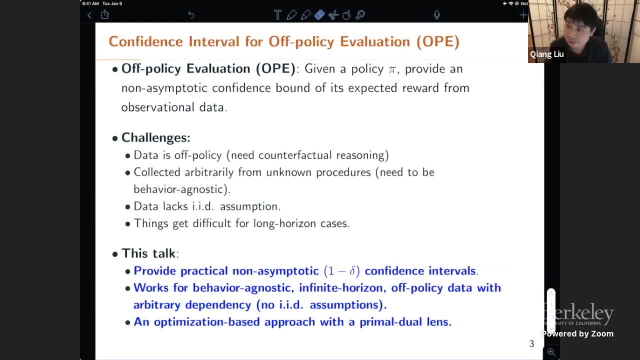 data with arbitrary dependencies. So it's very nice, flexible and again, the idea I will talk about that it's a kind of optimization view with sort of a primal-due flavor. Okay, so let's talk about the background. The setting is very simple and standard. 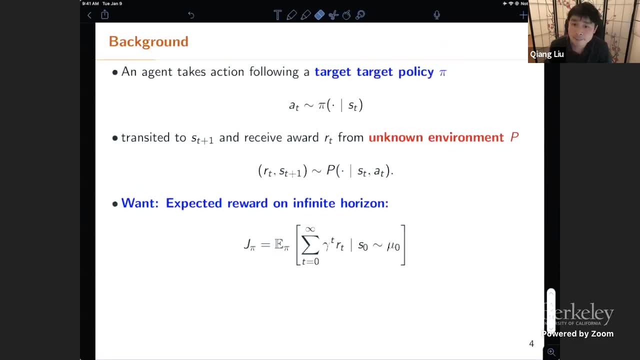 We have a tuck-in policy pie which is given: We have an unknown environment. p is unknown to us. So basically, every time the agent take action based on state and then based on the action state, you have an environment that transit into another state. 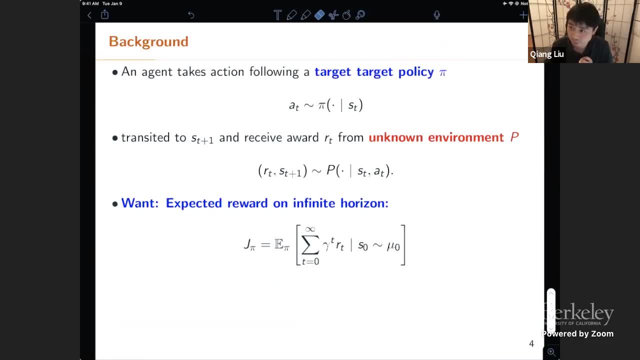 as t plus one. also we receive the reward. So both the way to receive the reward and the next state are unknown to the user, to the algorithm, And we want to estimate the expected reward over an infant horizon, which is something over all the time up to infinite, and of the reward discounted by a factor gamma t. 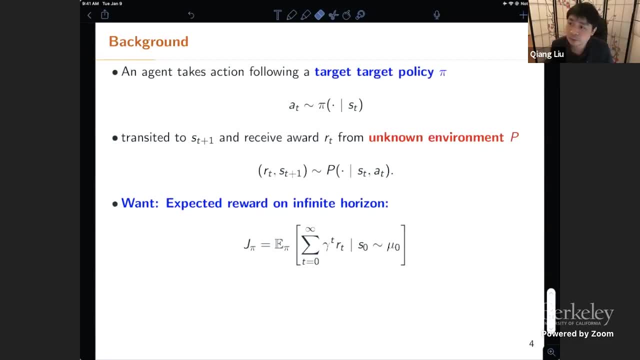 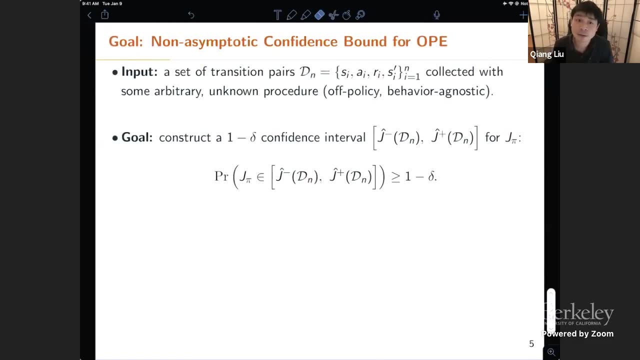 starting from some initialization. mu zero- Assume- here we assume mu zero is fixed- is known as well. Okay, so now the problem is given. in reality we don't know the true model, so we assume that we have transition pairs so I can actually label. So we have a collection of transition pairs. 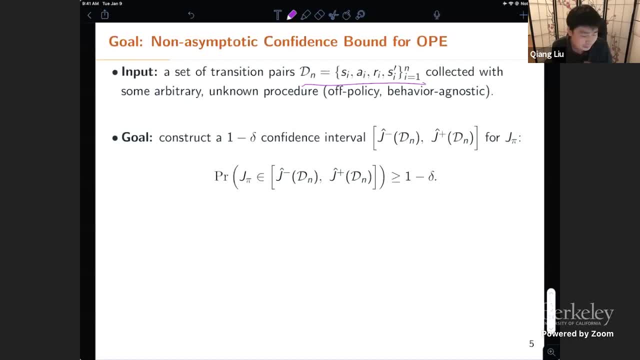 I will talk about what's the condition of the transition pairs. but basically we observe a bunch of things, a data set and then we want to construct the confidence interval, which is a function of the data, such that the probability that the confidence interval catch. 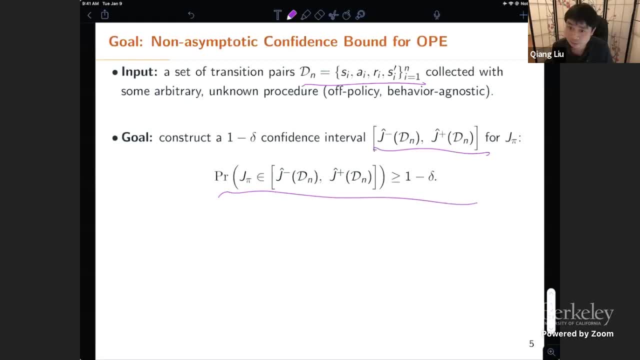 that the true value, the true expected reward, is larger than one minus delta. Delta is a confidence level, right? So here the probability is taken with respect to the randomness of data, right? So the interval is a standard confidence interval thing. So the interval is a random number. 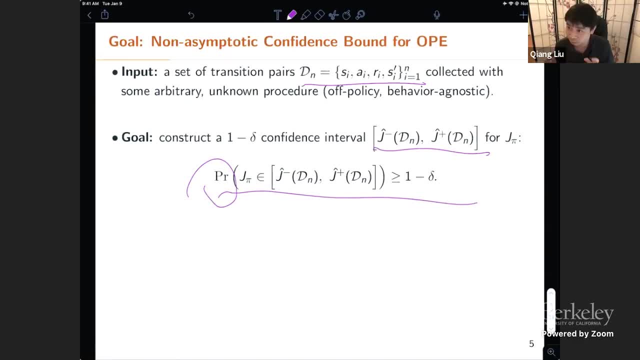 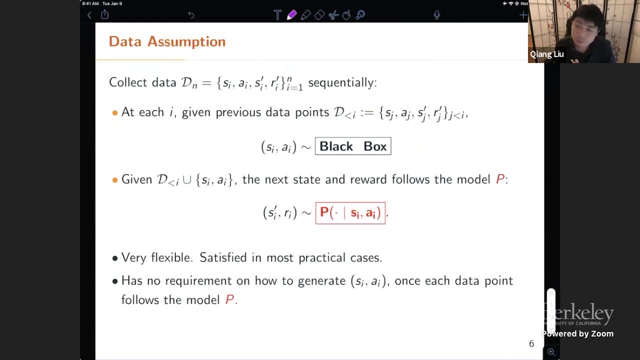 versus the true reward is a fixed, but want to make sure the interval actually catch the true value with high probability, right. Okay, so this is our formal definition of the data assumption. It's actually a very mild assumption, So the idea is that we assume we collected. 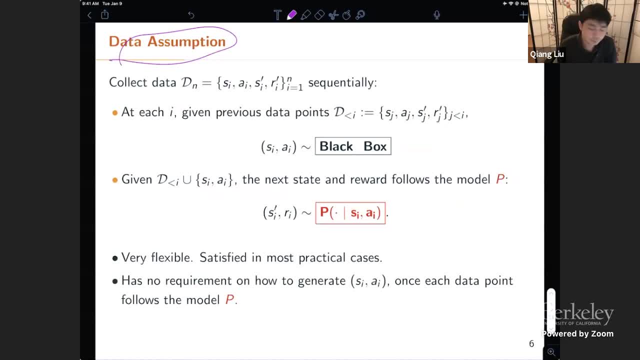 a set of transition pairs, right, And we assume the transition pairs are collected sequentially such that for each data point- I, the SA, the state and action is collected by some arbitrary procedure that is unknown. That is unknown to us given the previous data points. 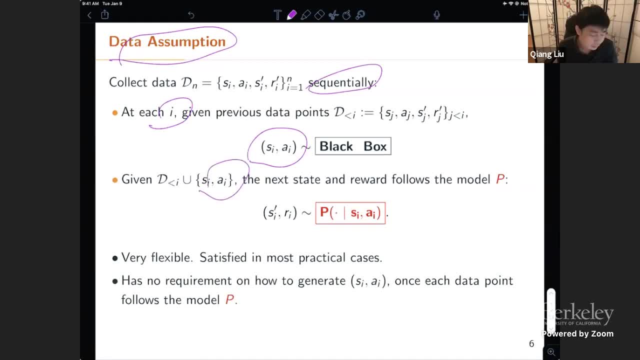 And then and then, given the state of the action pair, the next state, the next action, the next state and the reward is collected from the unknown true model right. So, really, the requirement, the only requirement we have, is that the next state and the reward. 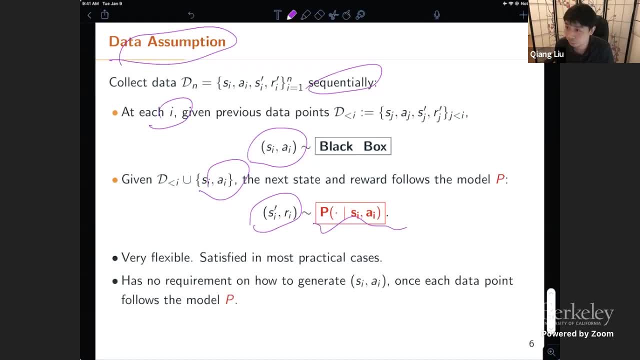 given the previous state and action has to follow the model, the true, the underlying and the non-dual environment, But otherwise it can be arbitrary. So the state action could be. you could use it in any way to decide your SA at each time. 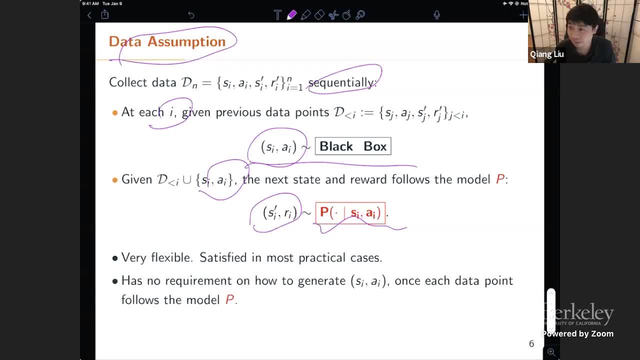 So. so it's very flexible. In fact, I cannot figure out a case when this is not satisfied. The only case I can figure out is when somehow that's a loopy dependency where you can travel back to time, but that's, that's doesn't seem to be realistic. 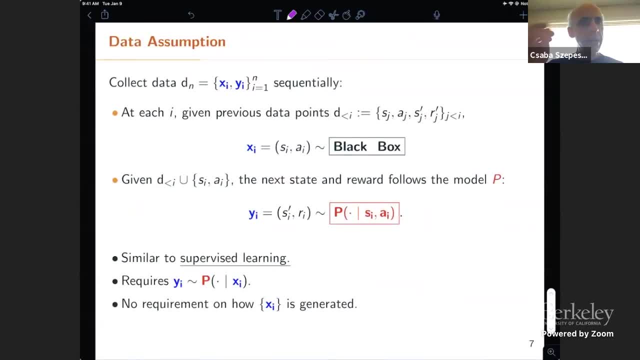 So just a second On this assumption. a quick question. So you say that this data is gathered sequentially with this black box, but it's not very clear to me whether you're assuming that this topos would be independent of each other. 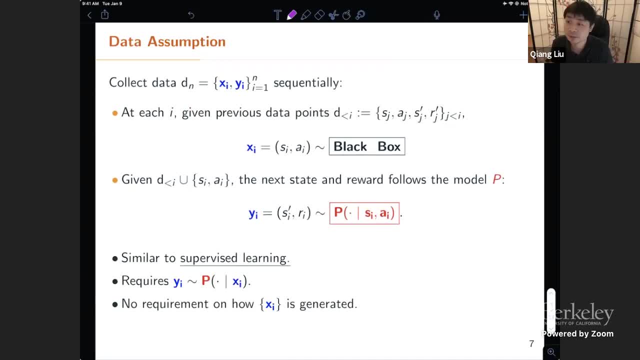 So this is a sequential process, right? You can think of it as a model And so like: is there going to be some mixing assumption here? No, just no mixing assumption. That's the key, right? So maybe I will, I think on this slide. 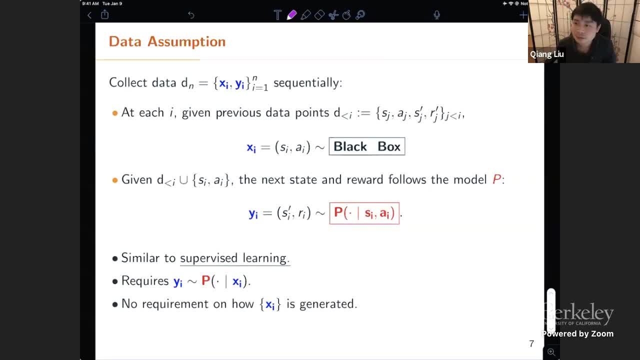 it will make it very, very clear, Much clear. So the idea is that you can kind of view this as a two-part setting. I think this is really a kind of a two-part setting. I think I got it Like you're going to use the assumption. 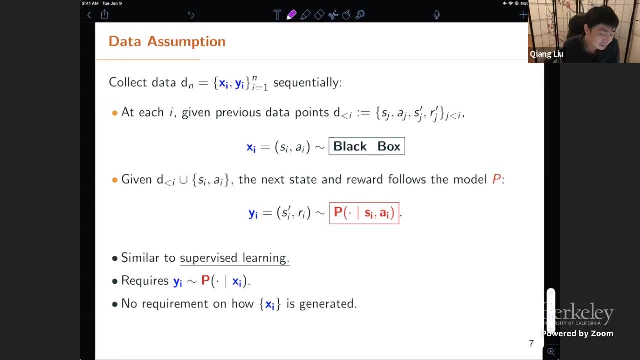 Yeah, yeah, yeah, yeah, yeah. So basically you can view SA as your feature, right, And then your Y as your label, right. So it's like a supervising. You want to give me X, you want to put in Y. 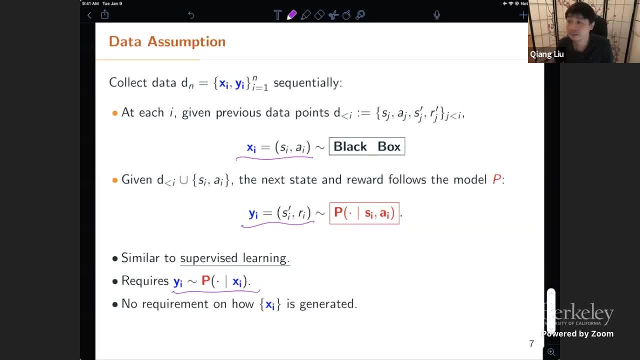 And really what I'm assuming is that Y, given X, follows the model. but then I don't assume anything about the data right. The data is collected arbitrary. This is really kind of a kind of a supervising learning setting. We really don't need to assume what the data comes from. 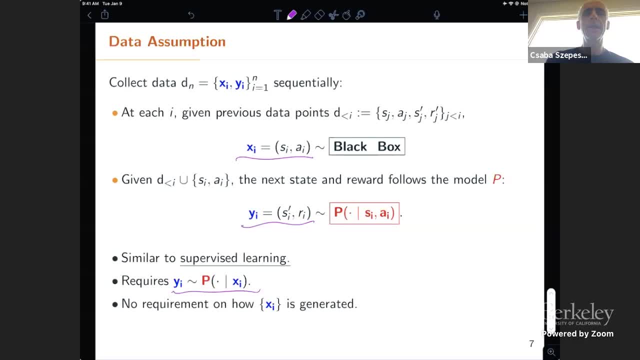 Even more general right. So the question I'm asking whether the XIs could be sequentially correlated like the black box. Yeah, sequentially correlated. They could be deterministic, They could be arbitrary. The black box might decide, for example. 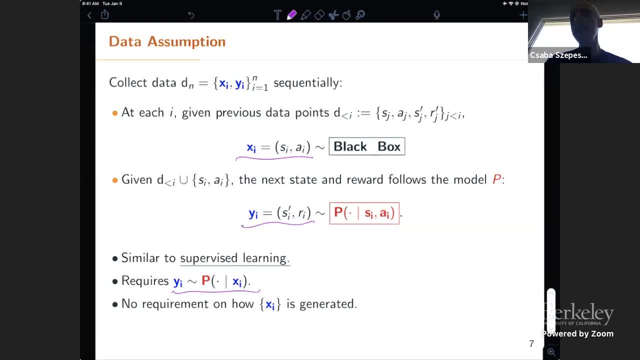 that I like this previous XI. Let's just go back and let's pick that again and hundred times more and stuff like that, Right, Yeah, Okay, yeah, Sounds great. So, yeah, the point again. I think the point is that the data is really arbitrary, right. 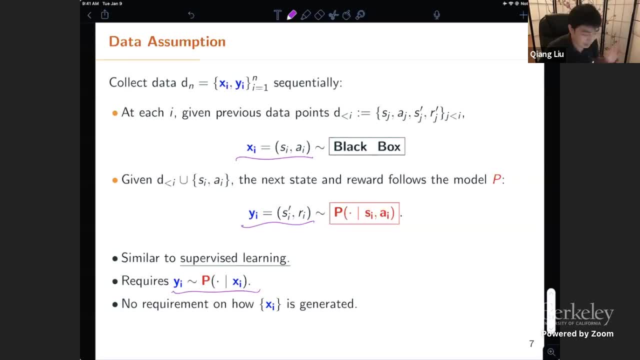 So XI could be dependent in some arbitrary fashion. The idea is that when we want to construct a confidence bound, we really don't care about how the data was generated. We only care about the information that data is carried to me right. So like when you generate data. 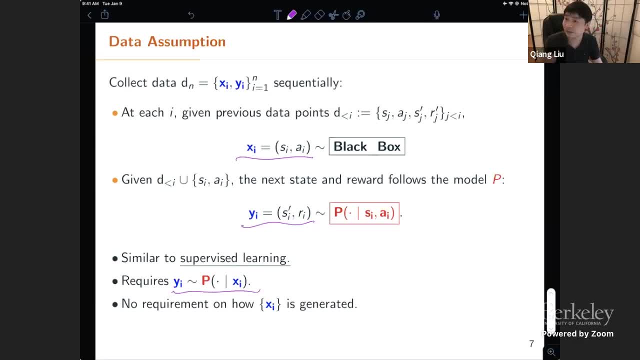 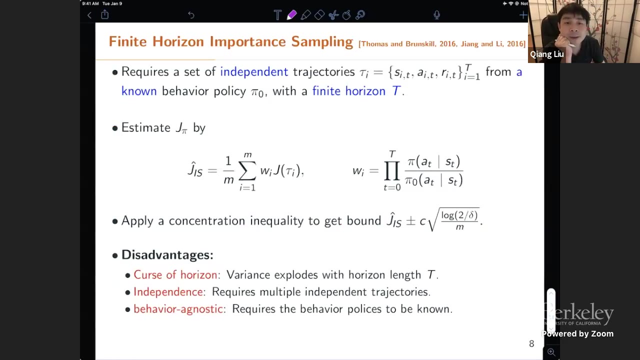 you have all kinds of assumptions, right, But once you get the data, the data is fixed right. So we don't need to care about how the data was generated, because by the time the data is given, it's already deterministic. Okay, so a traditional way to construct non asymptotic data. 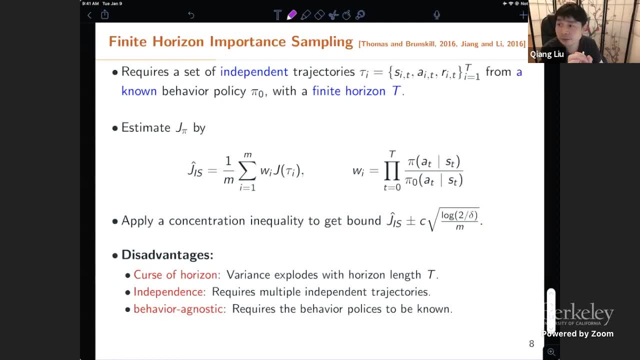 in confidence bounds. it seems that the only way to do this is using importance, sampling past constitutional inequalities. That's a larger, very classical literature on this, Many of the people here contributing heavily on this topic, And the idea is that you collect a set. 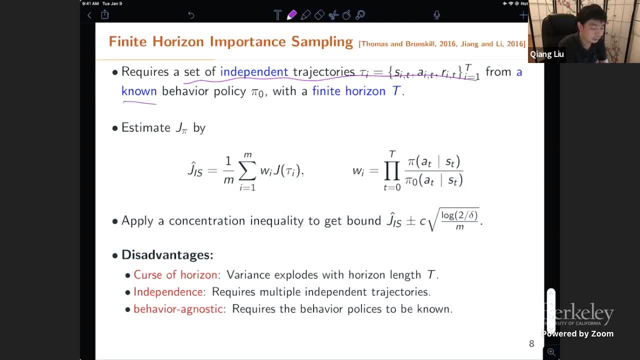 of independent trajectories from some non behavior policy pi zero. In this case, You have to have multiple trajectories that are independent, and you have to. the trajectory has to be drawn from some known policy pie. So it's not arbitrary dependency, right. it doesn't follow the assumption that I just mentioned and also it's not behavior agnostic, right. 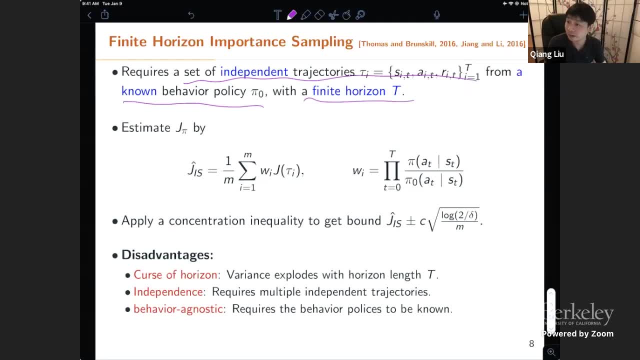 And also you have to truncate the horizons to be some finite horizon. In this case you can use a standard, important sampling estimator and basically design weights on the trajectories and then you can get a concentration bound using non-synthetic bound, using any constitution equality. So obviously there are lots of. 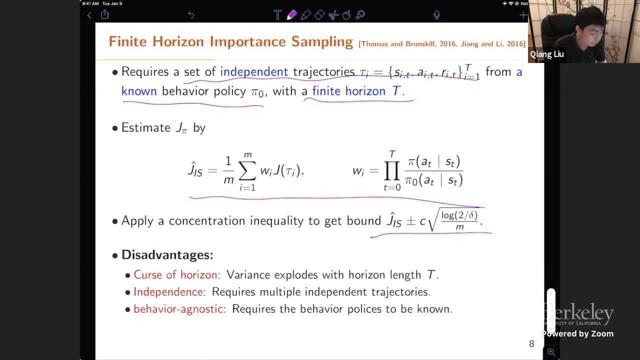 drawbacks? right, it doesn't. so actually it doesn't have the efficiency. So when you have a large horizon, T, this algorithm actually tends to degenerate. That's because your importance weight is a product. over the time. As you have lots of time, time goes to infinite. the variance of your importance weights grow exponentially. So that's very bad. There's something we call 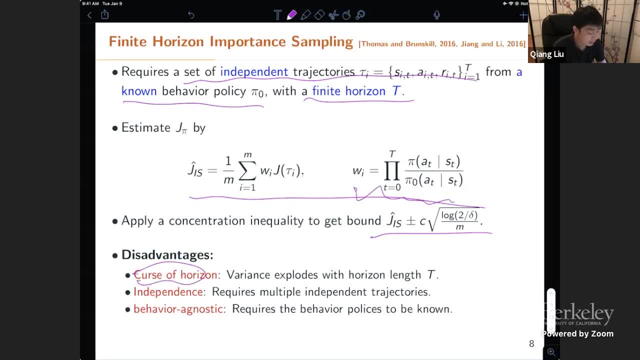 a causal horizon And also this algorithm has to require independent assumptions between the trajectories. If you don't have independent assumption, you can still give an estimation, but you cannot provide non-synthetic bound without providing a bound over the mixing coefficient of the Markov. 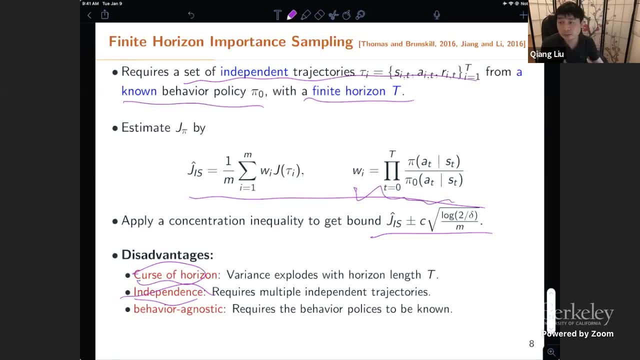 Asked, right. So as I want to emphasize here is that our algorithm doesn't require the mixing condition And also it's not behavioural plastic, right? so it doesn't work for our case. There are obviously many other ways to get confidence bounds for of policy, So there are bootstrap algorithms. 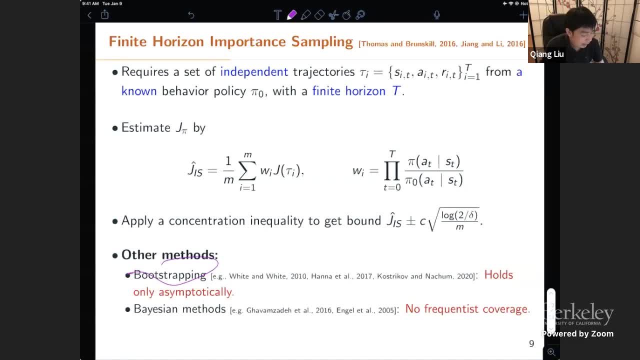 developed recently. Scott also had a work on this. But bootstrap is an asymptotic algorithm so it doesn't give non asymptotic guarantees. If we care about safety, we should go with non asymptotic, because that's a real guarantee And there are also Bayesian methods. 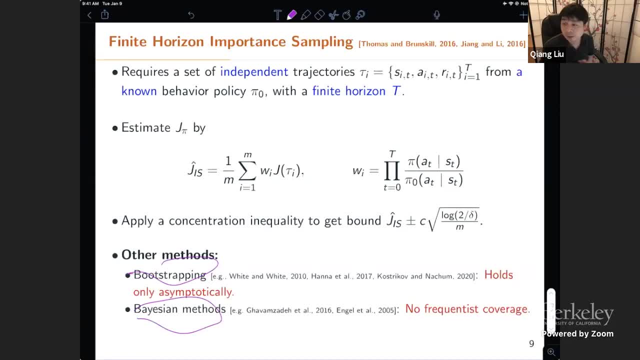 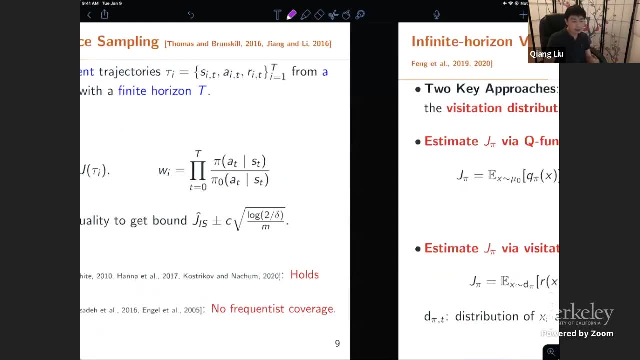 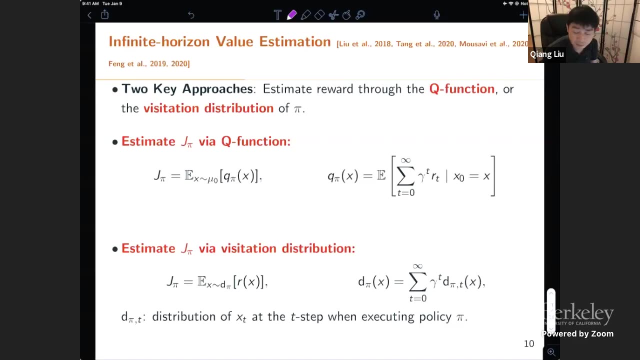 that quantify uncertainty in reinforced learning. but Bayesian doesn't have frequentist coverage, so it doesn't have the kind of guarantee that we want. Okay, so how do we solve this problem? Well, it starts from a line of work that I was getting to, together with Lee Hong and many other. 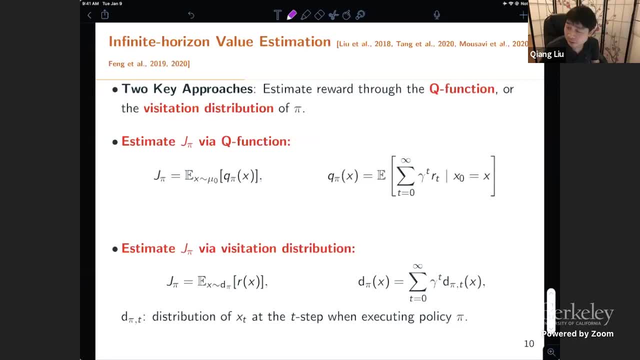 collaborators on infant horizon value estimation. So we have a sequence of work on estimating the reward without, first of all without a confidence estimation for the infant horizon case, when you have the cursor horizon for importance sampling, And then we talk about, and then this sort of work gradually moved towards to confidence estimation. But 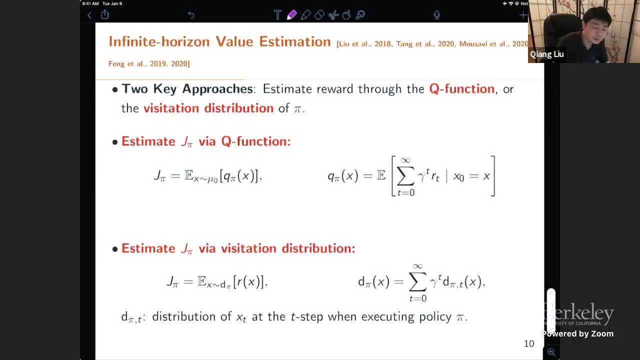 it more or less provides a foundation for my method, So I want to introduce this line of work. So it turns out that there are two major algorithms for infant horizon value estimation. One is based on Q function, another is based on visitation distribution. 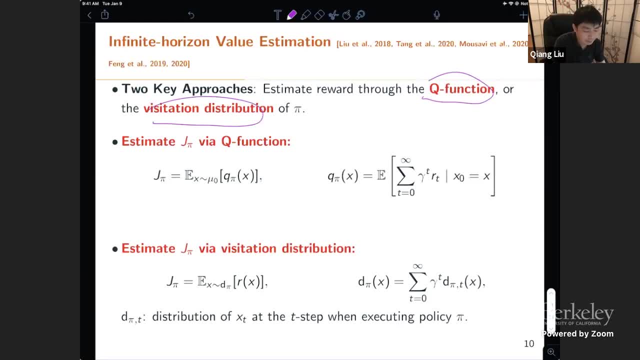 So the Q function idea is very simple. Basically, if you can estimate the Q function of the policy, the Q function is the cumulative reward, given that you start from a fixed state of action pair, where here I'm using X to represent the state of action pairs. 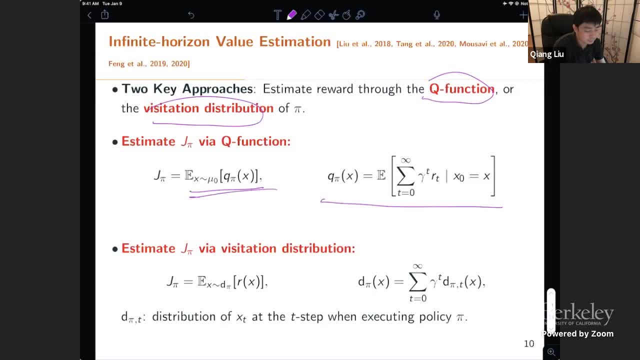 Then you can, if you know the Q function, you can just take the average expectation of your Q function over the initialization, over the initial states. That will give you your expected reward. This is one way to kind of think about expected reward. Another way to think about the reward is: 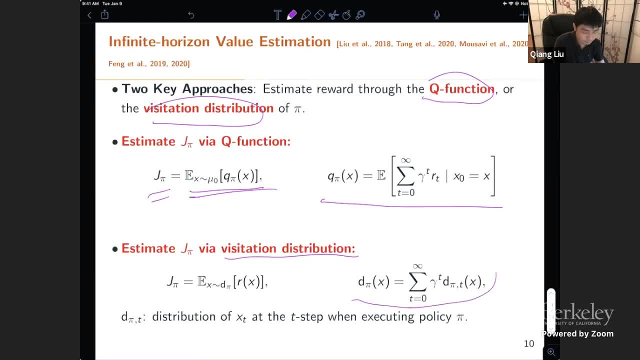 that you can calculate what's called the visitation distribution, which is the discounted average of the distribution of the states across time. So here, dpi t is the distribution of Xt. If you run the policy pi for t steps, starting from initialization, then you can get the estimation as well. 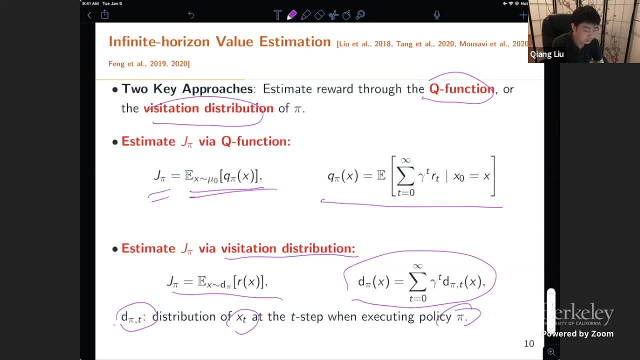 So the expected reward is going to be the expectation of the local reward taking expectation on the dpi. So you can sort of see these two ways, different ways to calculate the expected reward. They're really just, they are duality to each other. 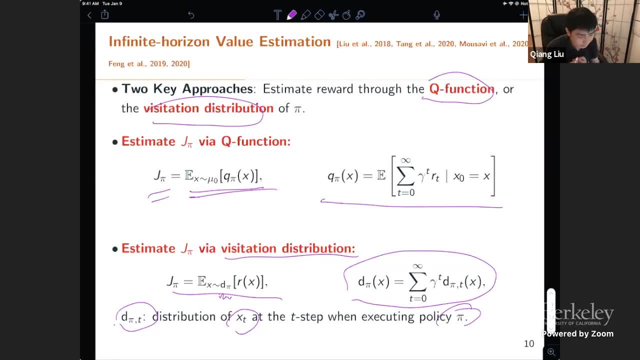 They have a prime or dual relation. I will talk about this. Many people also observed that, But I think the difference is really that when you talk about this summation over infinite right, So when you have this Q function representation, the summation is pushing inside the reward. 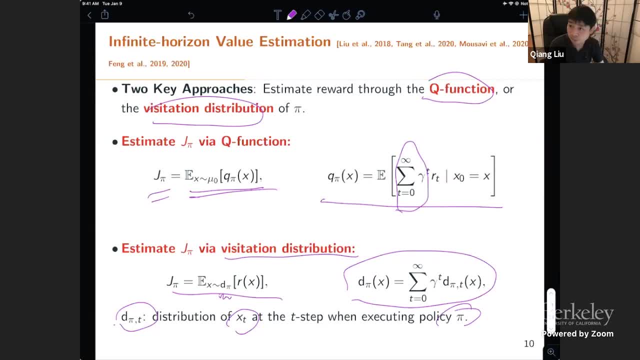 versus when you have the visitation distribution. the summation is pushed into the probability. The two ways to kind of counter summation. Okay, but then if we can estimate either with visitation distribution or Q function, we can construct our estimation. 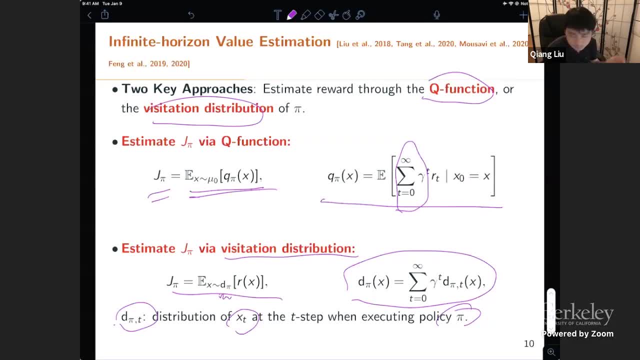 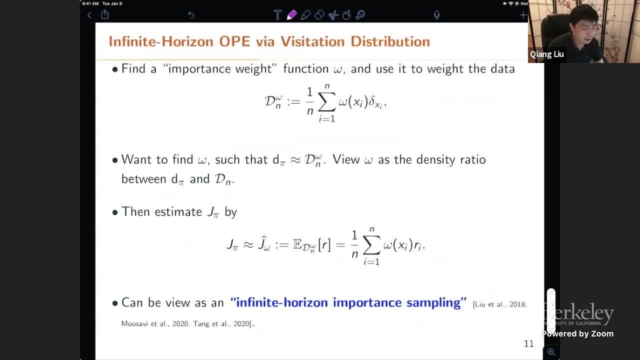 If we can, actually most we can use, we can do W vast estimation. Okay, so how to estimate visitation distribution? Well, we have this idea that you can actually put some importance weight on the data point. So here W is some weight distribution over the data points. 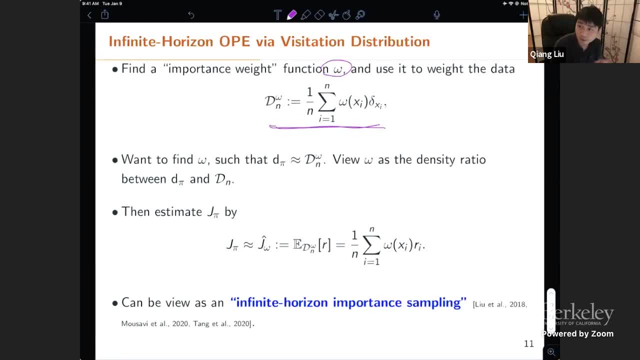 We can actually define this weighted empirical distribution over the distribution, where each data point is assigned with a weight, And then we want to find the weight such that the weighted distribution of the data actually follow matches the visitation distribution. right, If we can do this, then we can approximate. 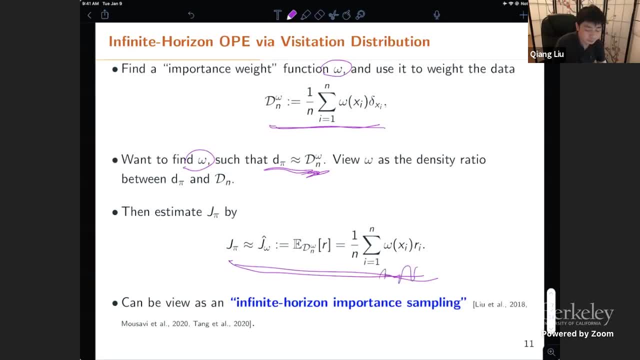 approximate the expected reward using the weighted sum over the reward, over the data set, right. So this is kind of like important sampling. but we are applying important sampling on the transition level and it's for infant horizon. So the importance: weight W here. 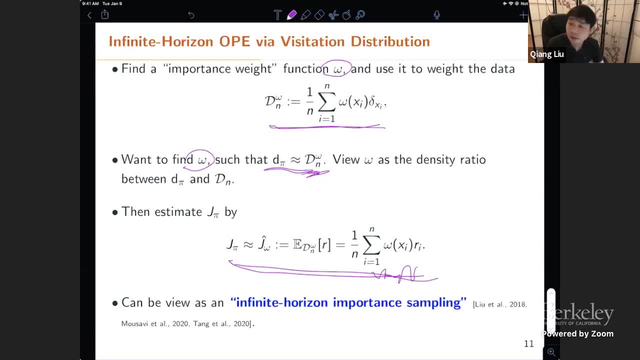 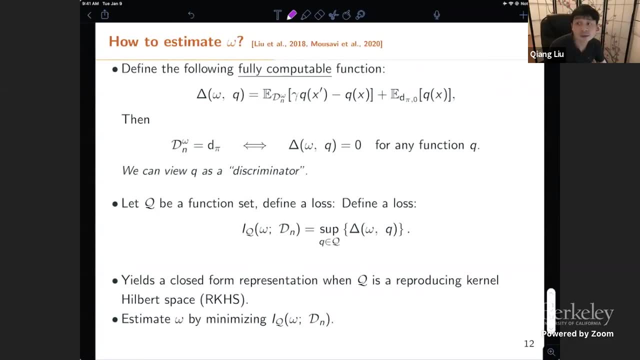 doesn't have a closed form solution, doesn't have a closed form representation, And we actually need to estimate it using optimization methods, right, But the way we estimate it is to define a reward function. The reward function we define it is a minimax reward. 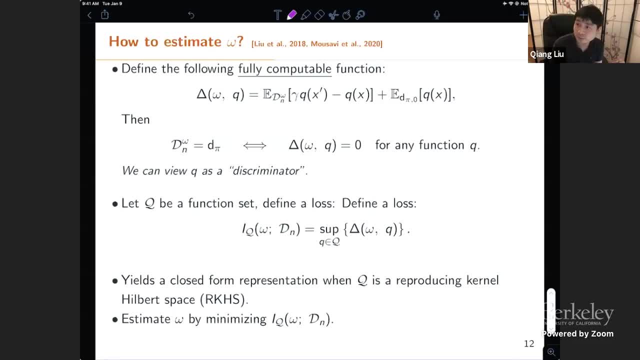 So the idea is that. so, basically, if you assume that the policy for giving the policy, that's Markov chain, where you essentially you are trying to estimate the stationary distribution of the Markov chain, and then what you can do is you write down: 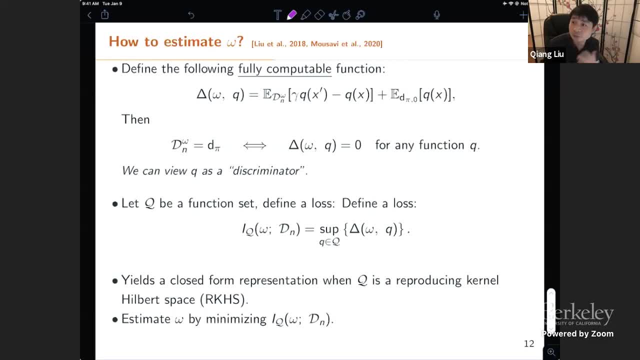 the fixed point equation for the Markov chain and we for reframe it a little bit. it turns out that you can show that we can define this delta function. I don't want to get into detail about what this function does, but basically this is a function that is fully computable. 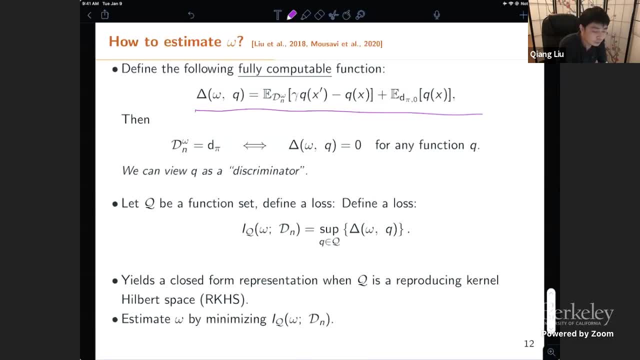 You can directly calculate it from the data and then you can show that this delta function equal to zero for n and q. here q is a kind of a discriminator function that we introduce, such that if w, if the dw, is exactly equal to the d pi. 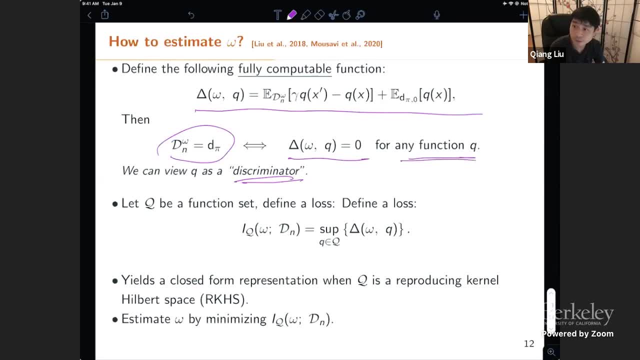 then this delta, equal to zero for any distribution q right, So quantifies the deviation of delta to the kind of true delta, deviation of w to the true w right. So in this way we can define this worst case kind of loss. 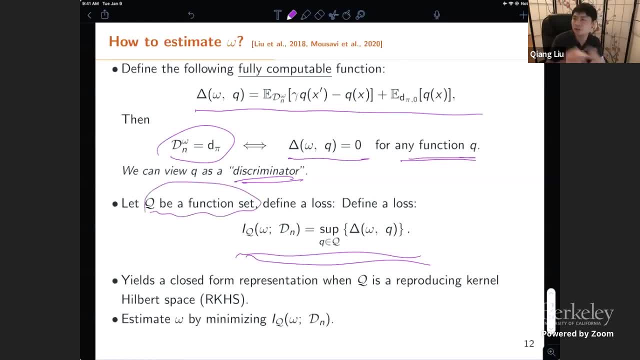 where you take a set of q function as a discriminator. It's kind of like a GAN style, where you find the worst case q right And if delta equal to zero for every q, then this loss function has to be zero. Otherwise it will be positive if the q is symmetric. 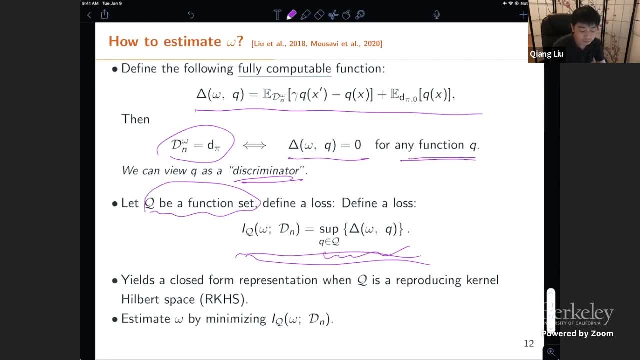 Then this defines a loss function. And if we, in addition, if we choose q to be a reproducing kernel- Hebrew space, it's a kernel space with a positive, definite kernel related to you think it's doing some kind of kernel regression. 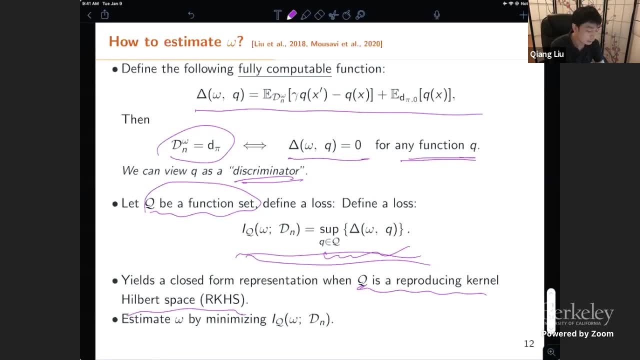 then you can actually write down the closed form solution for the loss function and you can minimize delta, minimize w to estimate, minimize the loss to estimate w, right? So that's a very quick overview of this idea, And- You have about four minutes left. 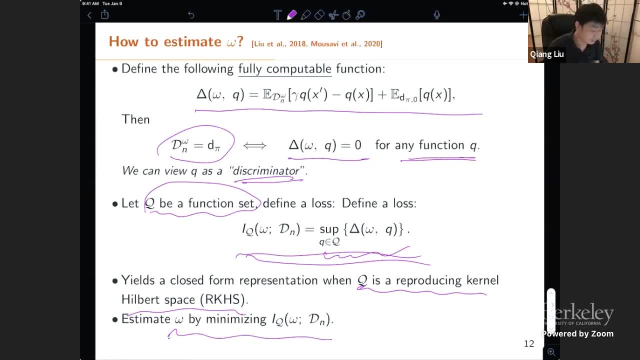 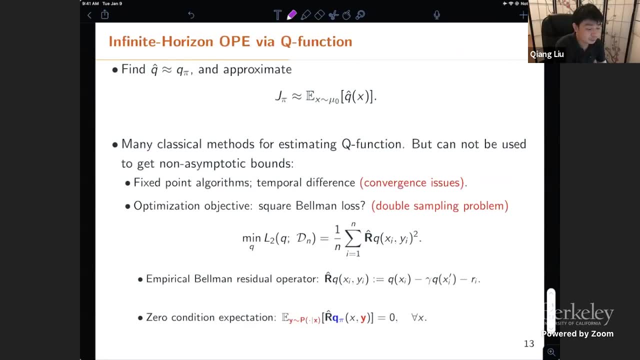 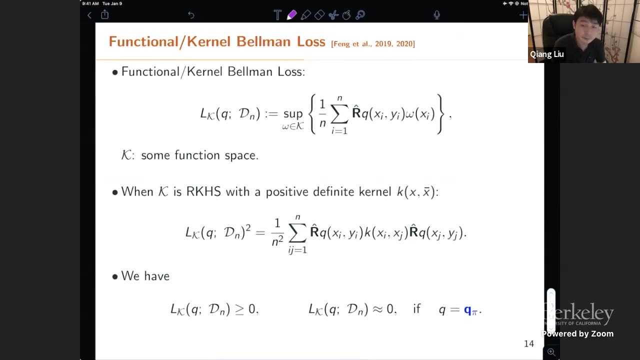 Sorry, You have about four minutes left. Oh, four minutes left, Okay, So I need to do really quick, Okay. So another approach is to do a q function estimation And again the idea is that we are going to introduce a kind of discrete loss. 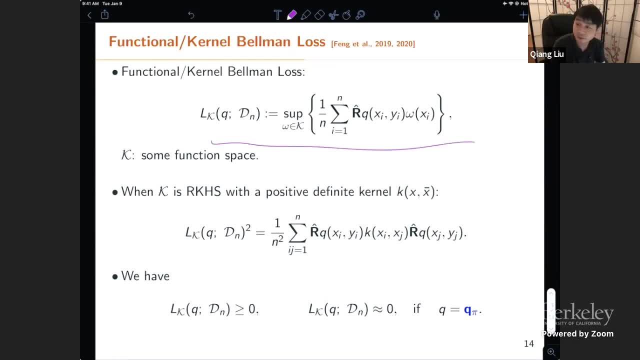 and the loss is defined in this way. We again, we use a minimax loss function to define the loss And again we introduce a discriminator function. If the discriminator function is a kernel, we can actually show that it has this code. 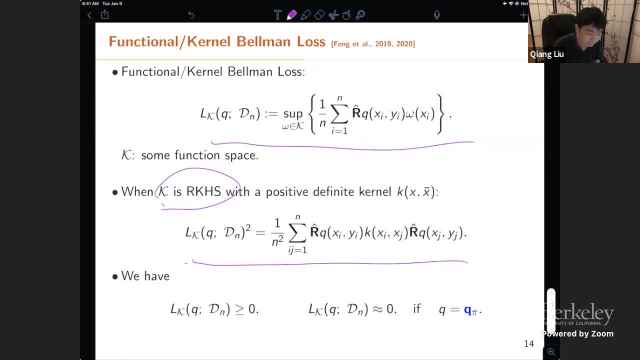 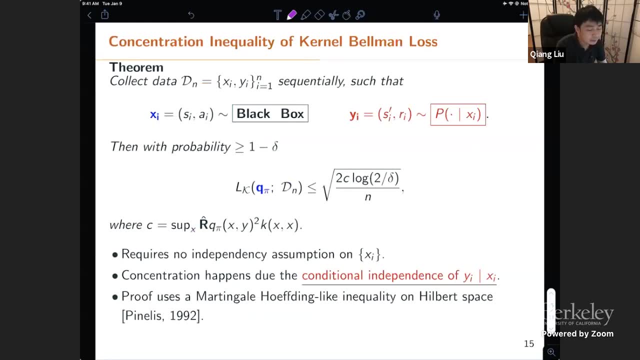 very nice closed form that can be calculated easily And the further. the key result that we have is that if the data is collected following the previous assumptions, then we can show that the kernel loss of the true q function is bounded by this non-isentotic bound. 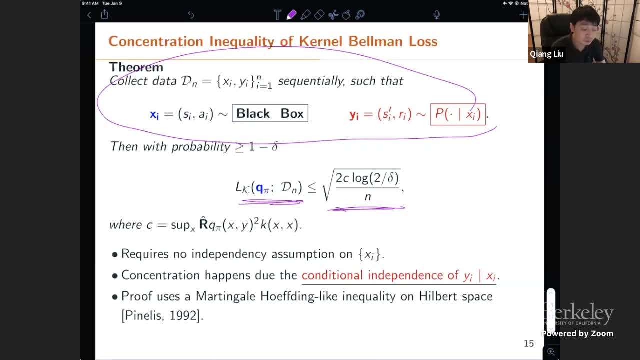 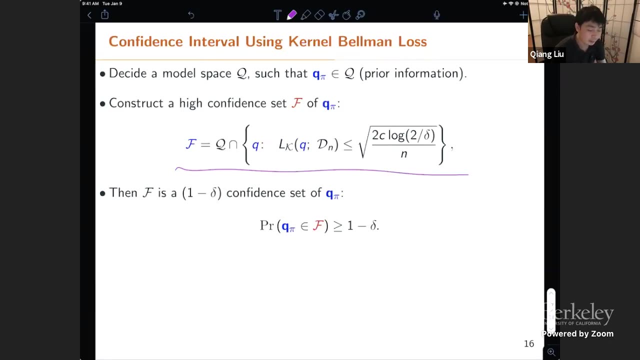 And this is important basically because the concentration equality actually doesn't require any sort of dependency among the independence of my exact. So, given this concentration inequality, what we can do is we can construct this concentration, this feasible region for q function right. 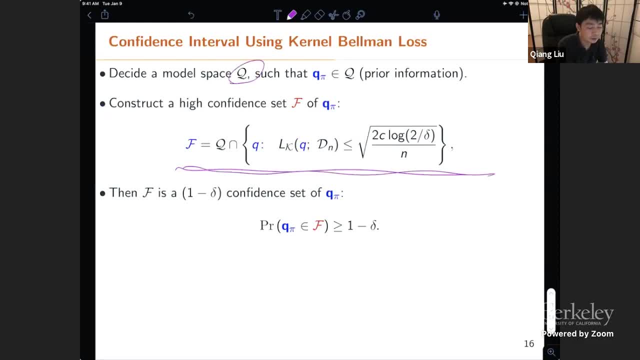 So if we define this function set where q is some model space, that is a prior information, that have captured q, q, pi, then this set has to be a confidence set for the true function right. It puts the non-isentotic guarantee. 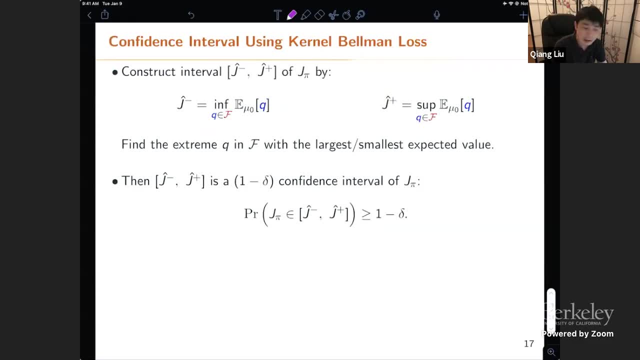 And then we can actually transform this feasible region of q- pi into a confidence interval for the expected reward by finding the extreme q functions. either maximize it, minimize it, we will get a confidence bound for the expected reward, And this frames optimization problem. 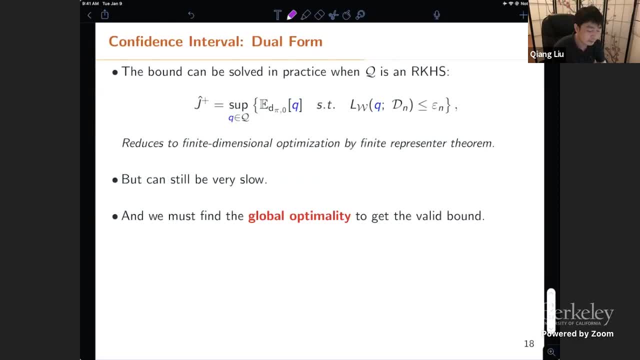 which can actually be solved in practice. but the disadvantage is that we have to solve this optimization to absolute global optimal in order to guarantee our methods. This is not ideal. So what we did was to divide a upper bound of this confidence interval. So the upper bound is a minimization problem. 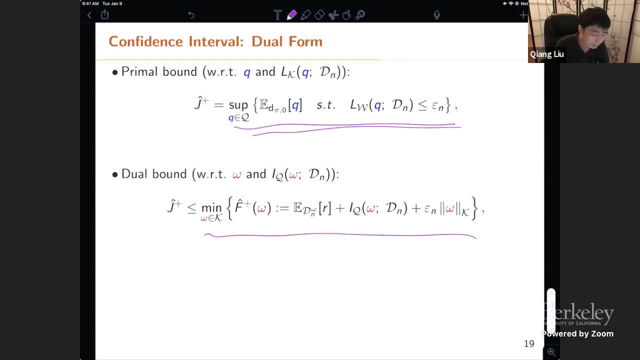 It's guaranteed to be larger than the bound that we have and depends on some w. In fact, if you look at it, the upper and lower bound has this very clear primal dual structure where the primal bound is framed as optimizing q function. 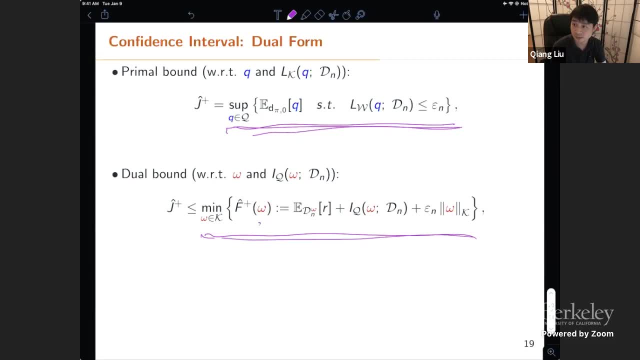 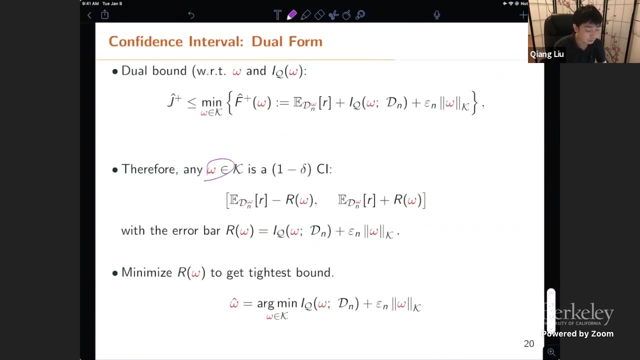 which is the dual bound, is actually framed as optimizing the density ratio. So in fact you can sort of see the kernel bound and loss for q, and here's the density, the loss for the density ratio as well, right, So now you can use for any w. 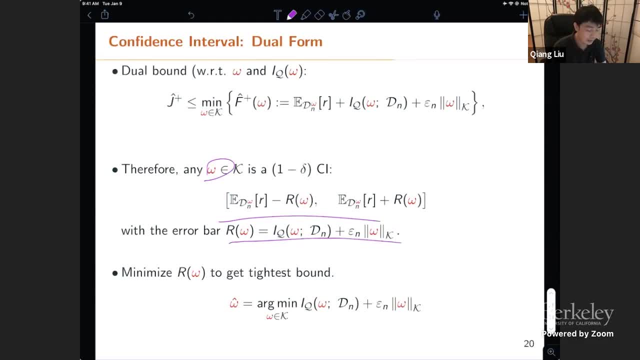 you can actually construct a confidence bound in this way. It's like assigning an error bar around, you know, around the density ratio estimation, and we can actually find the best w by minimizing the loss right. But in this case the idea is that you don't have to solve the thing. 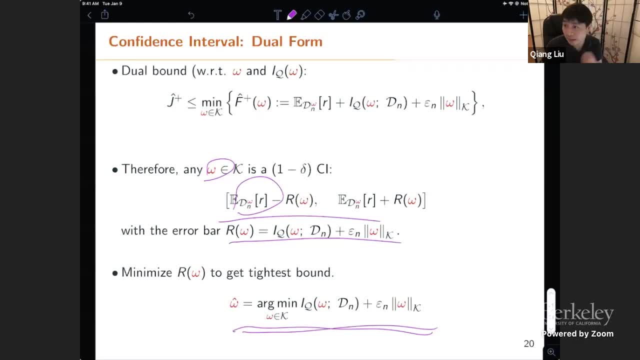 into global optimal solution. You just want to find whatever the best, because you will always guarantee the one delta condition. It's just that if you optimize delta, better you will get a tighter bound. Okay, so this is in fact our method. 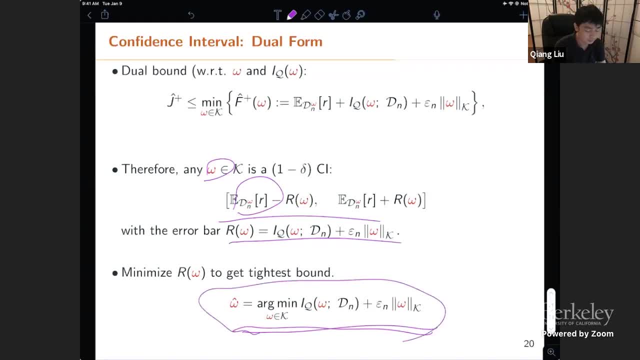 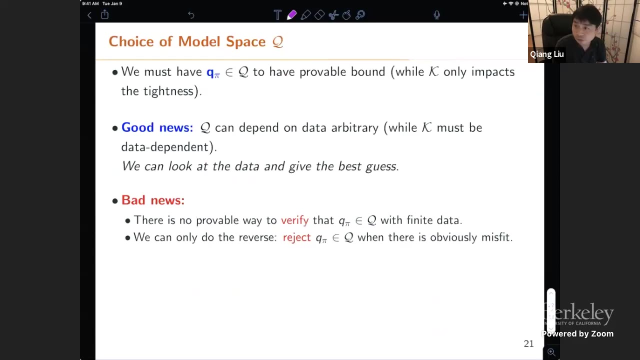 It's a very simple algorithm. So basically you use: find a density estimation, density ratio estimation by minimizing this loss. Try your best. You don't have to find the global optimal and then construct your bound in this way, right? So here's a few discussions. 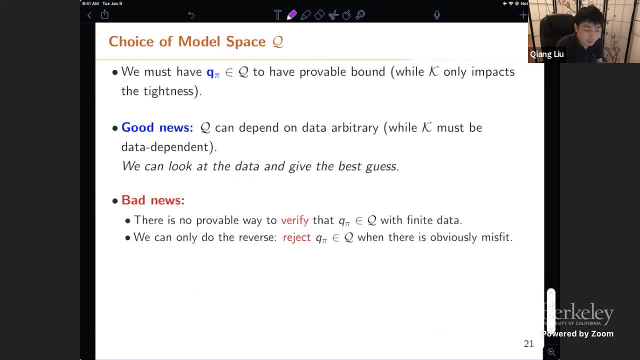 I'm not sure I will have time, but the idea is that our method actually critically- based on the assumption that the q function actually follows- belongs to a family, a model family. It's very similar to Shupai's learning, where we have to assume certain model family. 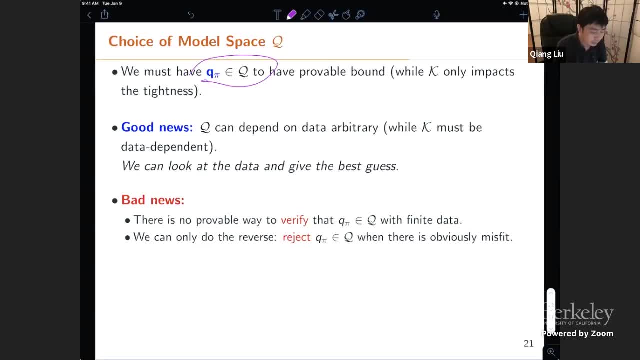 We cannot do statistics without any assumption. right, It turns out we cannot actually positively verify the assumptions. Again, it's the same thing as the statistics. Well, we cannot absolutely verify the model. assumptions We can reject, but we can never absolutely satisfy. 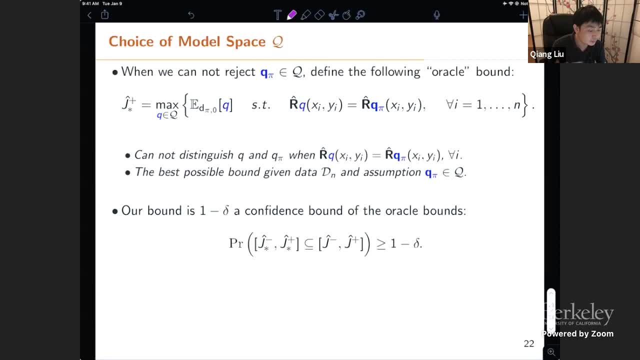 So that's a model miss specification problem And we can actually show that even if we cannot verify that assumption, we can still kind of interpret our methods as trying best, as trying to get up a bound of some kind of Oracle estimation that is accessible given the data. 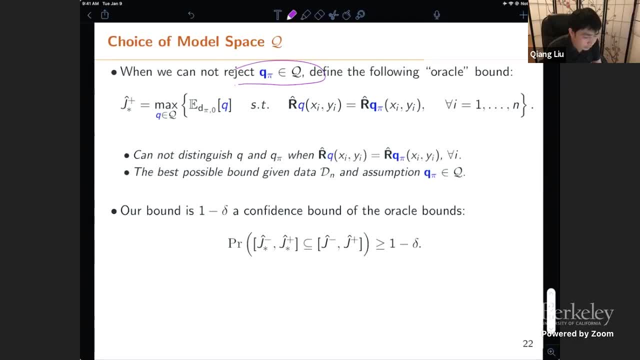 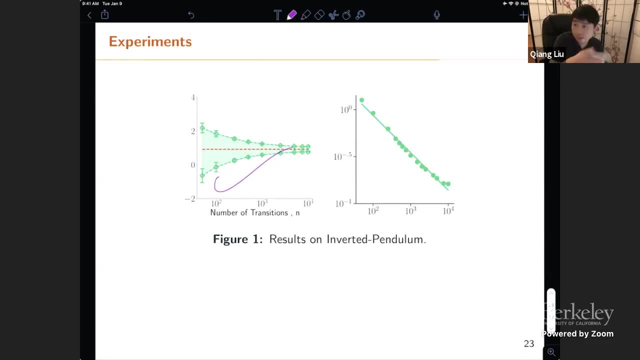 So I wouldn't get detail, but if that's a question, I can explain more. So we have some simple example here. So this is going to be what it looks like. If you check the gap, you can see that it looks like this. 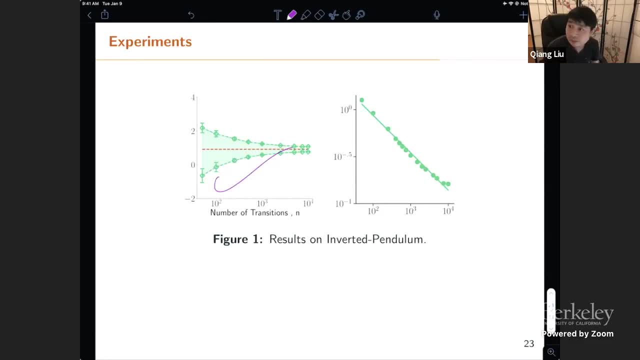 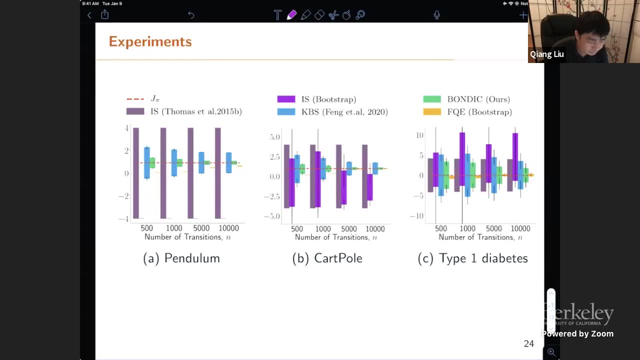 You can see the gap between the confidence intervals actually decays nicely with the data. So it's a consistent algorithm. These are a few comparisons with other methods. So basically what we observe is that: so the green line is our methods right. 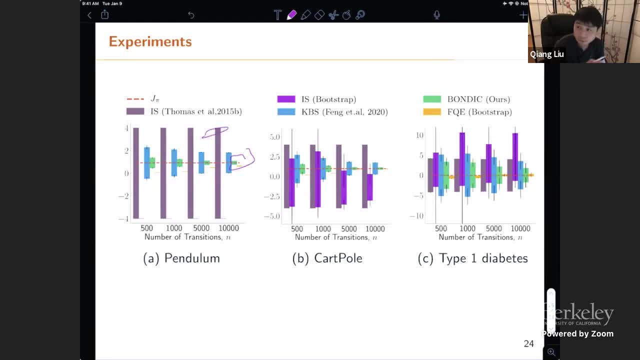 And if you use the important sampling with concentration bound, you will guarantee non-isotopics as well, but it will be much looser than our bound. And then if you use other methods, like the bootstrap for example, you cannot guarantee 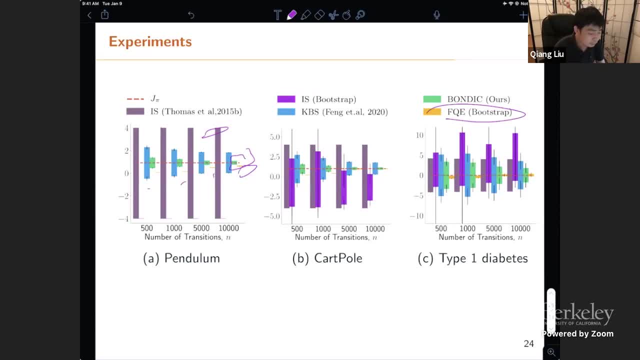 non-isotopic bound, so you will have the risk of not catching the true value, which is, if you have the non-isotopic guarantee, you can always, with hyper-B, catch the true values. Okay, so I'm stopping here. 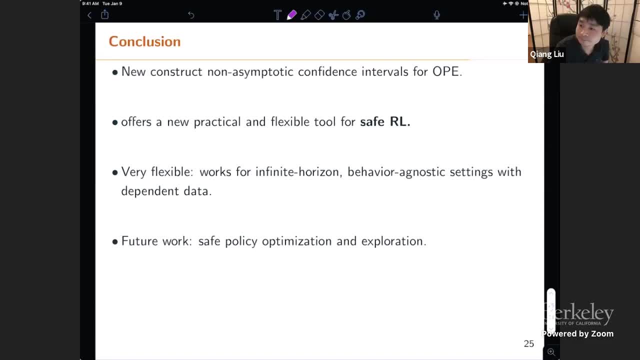 I'm sorry that this is over time. Thank you so much, Chiang. I think there was some discussion, some questions from Chaba about end-of-minute assumptions, So I'll open the floor for questions and we can start there. Yeah. 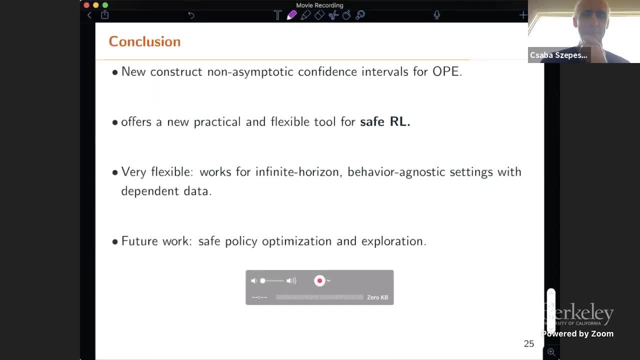 Hey, very, very nice. I read a paper a while ago and I kept confusing myself about multiple things. I guess, maybe at a very high level. you also said at the end is that this realizability is highly crucial, And what you're doing is that, rather than assuming, 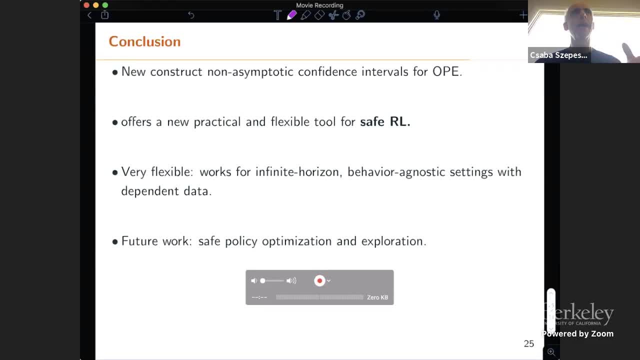 that you would estimate a model. you just assume that a function or features are given to you. maybe you can push it to infinite dimensional spaces, whatnot? but so you're given these features, or arcadia space, and you assume realizability. and that's the way you avoid the mixing assumption. 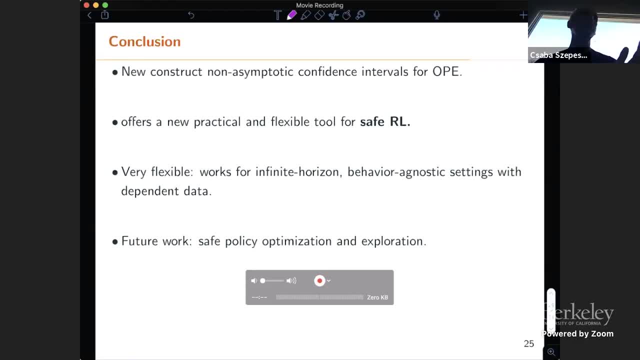 Exactly exactly. I'm basically Normally just estimate a model and then, based on the estimated model, you can evaluate any policy and then you can get confidence bonds with that way as well, by assuming realizability in a way. but this way are kind of like so you could do the same thing. what i want to say in linear mdps with chijin: 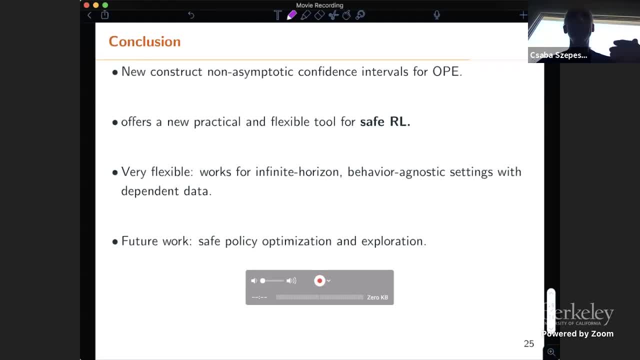 style: linear mdps, right, uh, but uh, then that's. that's a little bit stronger than the assumption that you're doing right. and then you kind of avoid estimating the mdp, go directly for us the action value function and you just show that everything like including confidence, intel was uh. 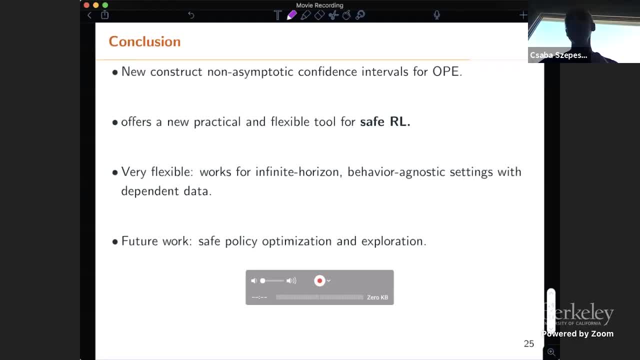 worked out, uh, super nicely, which is, which is very neat, all right. so with that, let's let's make this a question. uh, so do you have any thoughts about, like, what to do in the unrealizable setting? uh, how bad is that. i have some dark thoughts about that, uh, so what do you mean? so, do you mean? 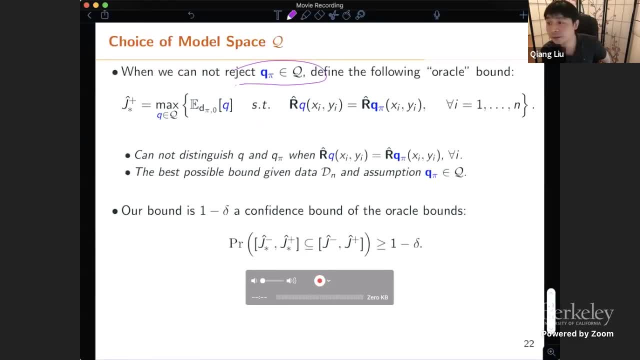 the case when the um, the model assumption, doesn't, uh, doesn't, doesn't satisfy, of course, yeah, yeah, well, so you? I think this is a very tricky question. Here's the thing, right, So we are taking the model of space to be a RKH space. 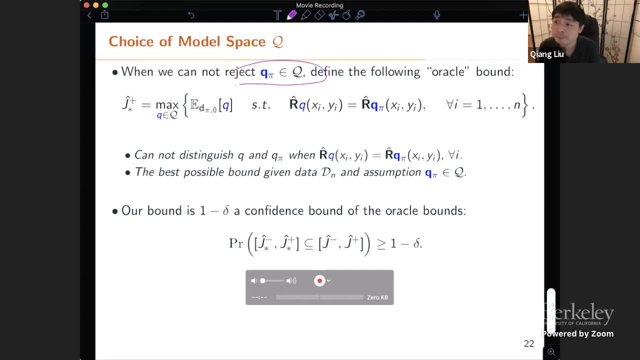 It's a kernel space, it's a infinite dimensional, So we can. so there will be two cases: One if the, so we have, the data is given And, as I mentioned here, we can. actually, this is a very special thing about this algorithm. 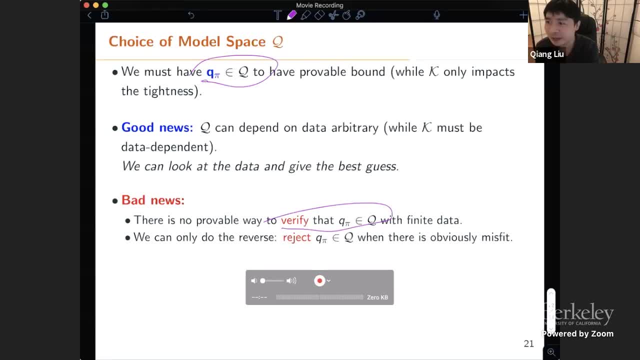 What we can do is we can take the data and just look at data very carefully, using any algorithm to figure out the queue, And the queue can actually depend on data in arbitrary way. This is unusual. This is what's different from the. So we can look at the data and construct a queue. 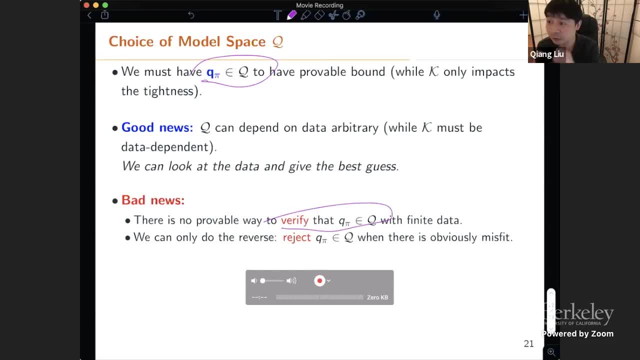 such that it's large enough, such that we cannot statistically reject the assumption. So there were no model misspecification in this case. The only difficulty here is that when I construct a very large queue such that I cannot reject my hypothesis, I can still 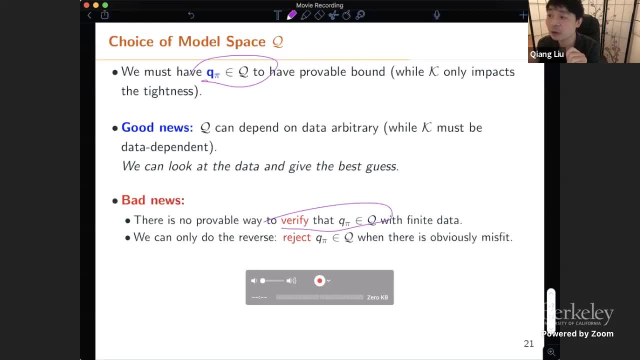 I can, I still cannot guarantee that my true queue will in fact be inside the queue that I have, Because this is. this is because the data assumption that we had earlier was really weak. We didn't assume anything about the distribution of the state. 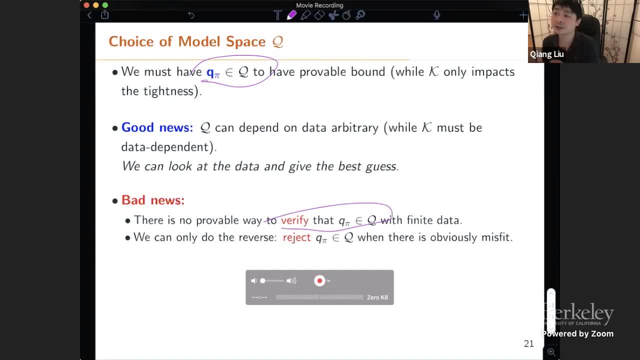 So because of this weak assumption, in fact statistically we cannot identify case reject, we cannot positively decide a case when queue is indeed in the model space. So we don't have the model misspecification problem, We, more like, have the model non-identifiability problem working. 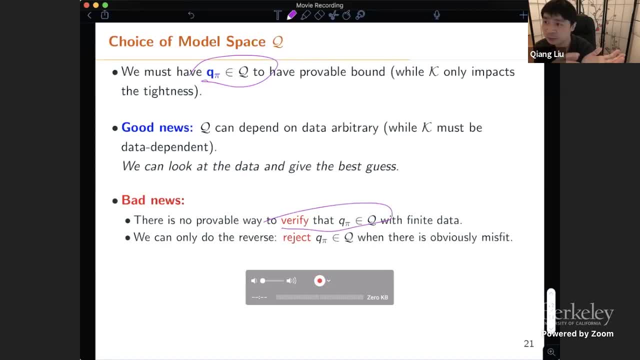 We cannot decide a model, set of models, given the information that we have, We fundamentally cannot decide the model. but it's not about the misspecification, Because if that's a misspecification we can actually reject that. How does rejection work exactly? 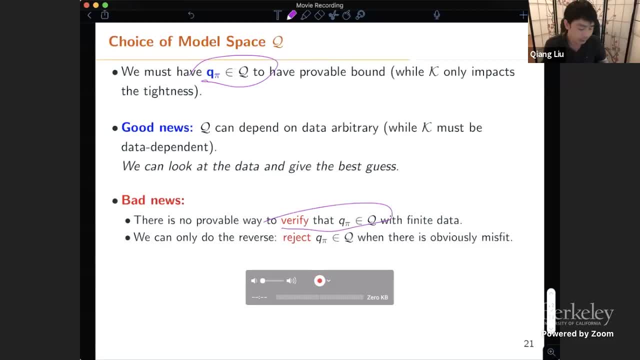 So rejection is that you can. you can calculate the loss function of the functions inside the queue, inside your distribution. And if all the queues- You're writing, so I can't see it. Yeah, Like you have to make that recording thing go away. 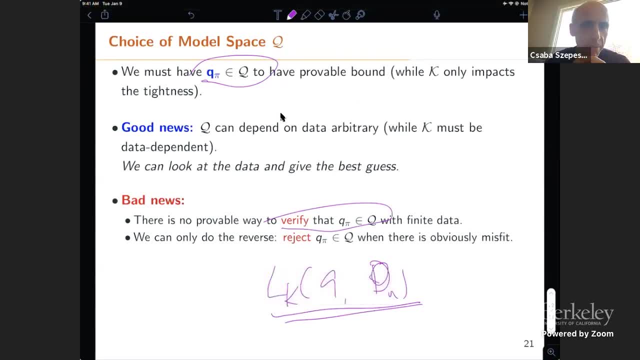 I don't know whether it's on everyone's screen, but I'd write some other point. Yeah right, Okay, good. Oh, okay, That's weird, Okay, Yes. So the idea is that you can calculate the kernel loss. 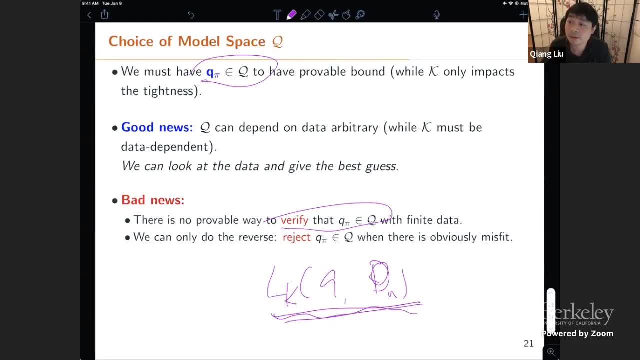 for every queue inside the model space And if every, if that lower bound is large is large, then it will reject Basically. if every data point, if every queue inside the function space has a large kernel loss, domain loss, then you reject it. 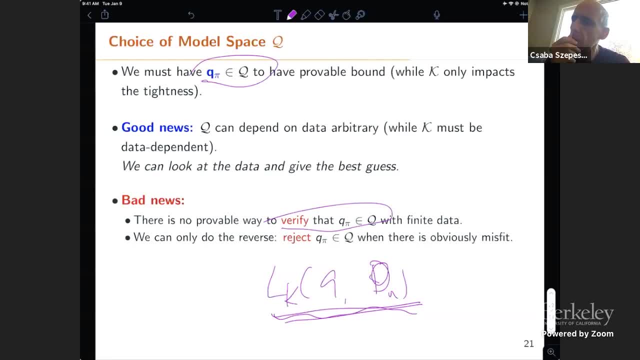 Okay, so you'll basically say that there is no way I can support the data with my function class. Then you say that my function class was not big enough. Is that ever going to happen if you have a universal Arcadia space? Yes, but the problem is the problem, right.